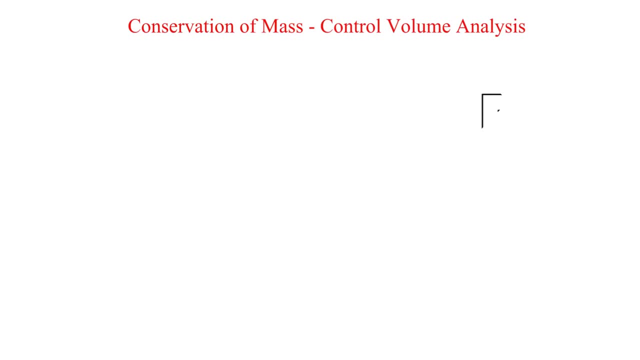 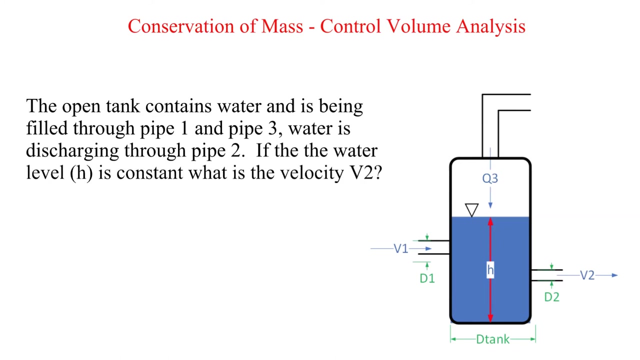 integration. Here is the problem statement and the corresponding diagram. The open tank contains water and is being filled through pipe 1 and pipe 3, water is discharging through pipe 2.. If the the water level H is constant, what is the velocity V2?? 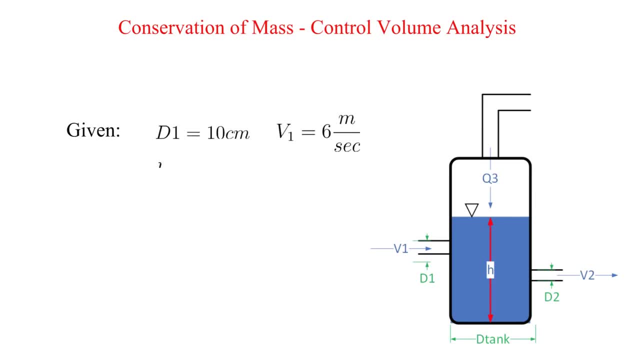 Below is the provided information. Now let's start solving the problem. Recall: we are trying to find the velocity at point 2.. We can use conservation of mass for a control volume. It is shown below. Let's start simplifying. If the water level in the tank H is constant, then it is steady state. 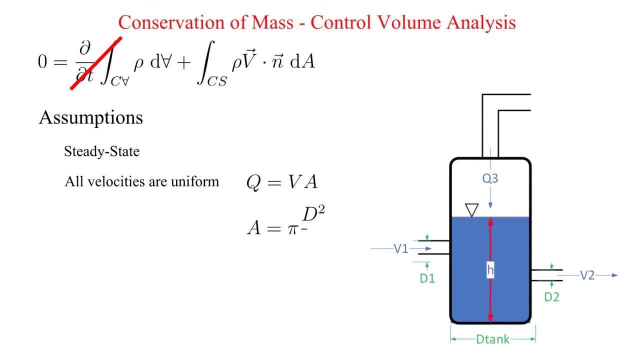 We will also use the definition of volumetric flow rate Q and how to calculate an area using the diameter. Next, we need to define the control volume. The conservation laws apply to any control volume. However, we must choose a control volume that allows us to solve the problem. 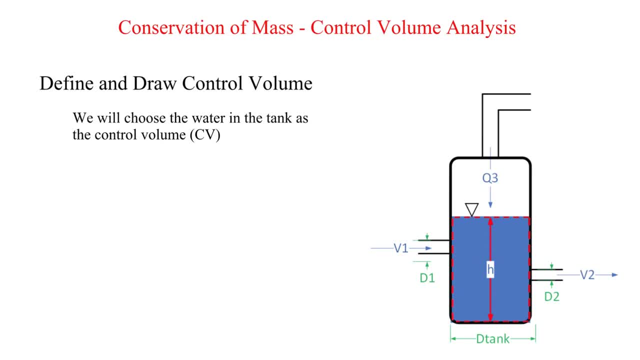 We will choose the water in the tank as the control volume. Next, we identify the surfaces where the mass flux is not zero. to simplify the surface integral, There are three. The integral conservation of mass equation expands as shown below. Let's review the dot function. 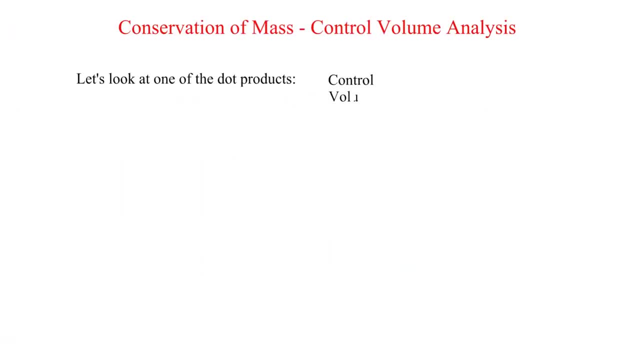 We will use the definition of volumetric flow rate Q and how to calculate an area using a control volume. Let's review the dot product in the surface integrals by looking closely at surface 1.. The unit normal vector is pointed out or away from the control volume. 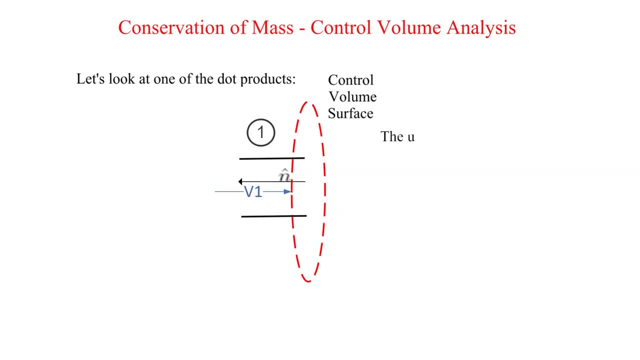 At this surface the velocity is coming into the control volume. The angle between the unit normal vector and the velocity vector is 180 degrees. The dot product returns a negative sign In conservation of mass for a fixed, non-deforming control volume. inflows are negative and outflows 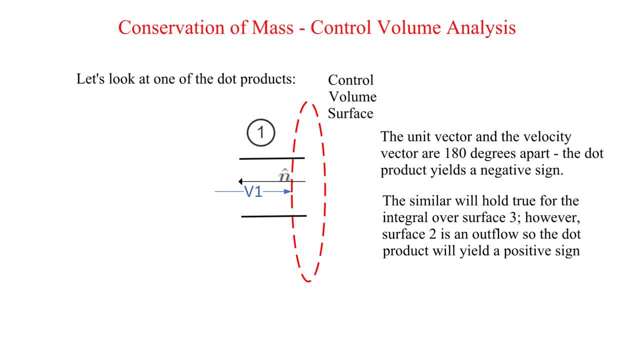 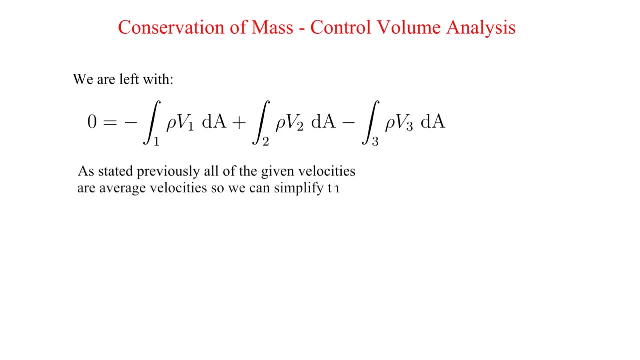 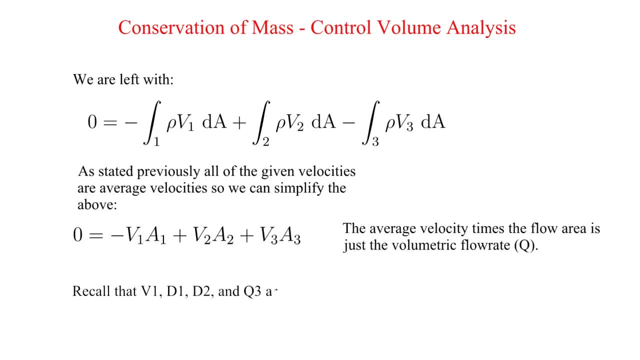 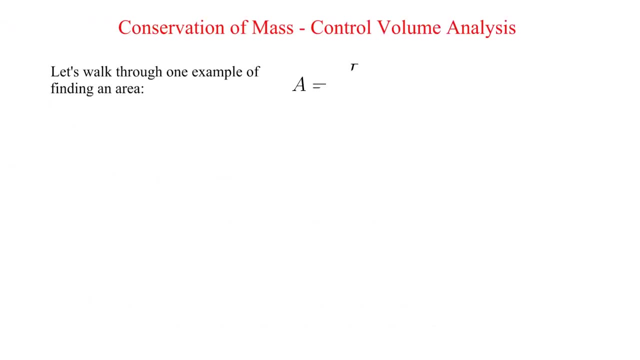 Recall that the average velocity times the flow area is just the volumetric flow rate q. Putting this together allows us to solve for the velocity at point 2, as shown below. Below is some arithmetic solving for areas 1 and 2 with the provided data.